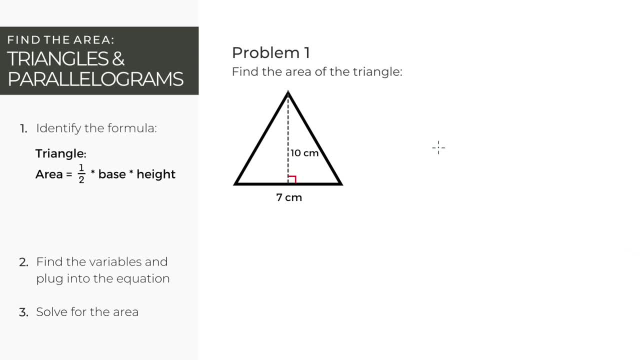 For a first step, we can actually use an equation that someone else a long, long time ago figured out for us: where the area of any triangle is one half times base times height, You might also see it written like this, with just letters. For our second step, let's look into what that equation 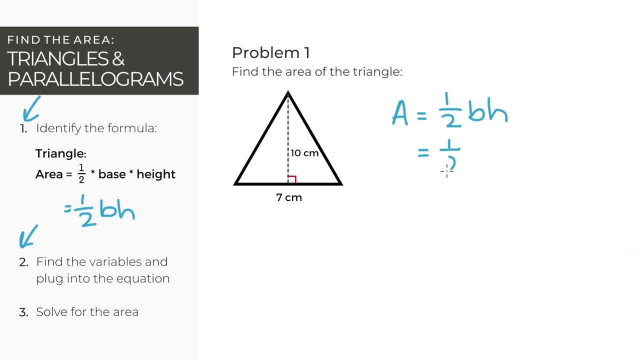 actually means When we say base. it's the length of this line. right here, You can think of the base as the side that the triangle is just sitting on, which, in this case, is 7- 7.. Now for the height. it's the length of this line. right here, You can think of the height as just how. 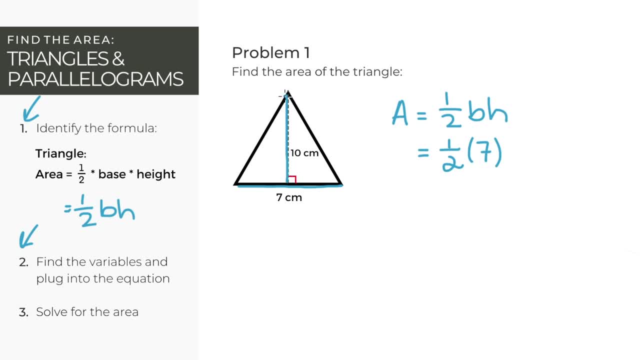 tall the triangle is. Just take a look at the point directly above the base and draw a straight line down and note that the lines for the base and height are always perpendicular to each other, meaning that they are always at a 90 degree angle. From this diagram we can tell that the height of 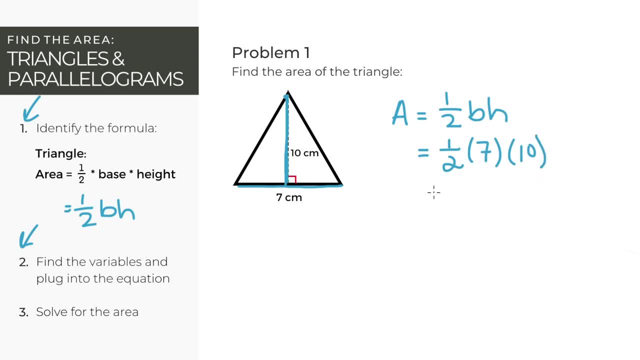 this triangle is 10 centimeters. For a third and final step, let's solve the equation. We have that the area of the triangle is equal to one half times the base, which is 7 centimeters, and the height, which is 10 centimeters. 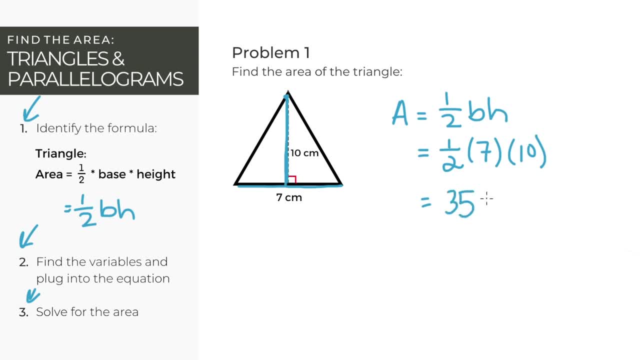 and we'll get 35 centimeters squared for the area of our triangle. And that's it. That's our answer. Let's try the same thing with a different looking triangle. For the first step, we're still using the same equation where the area of the triangle is one half base times height. 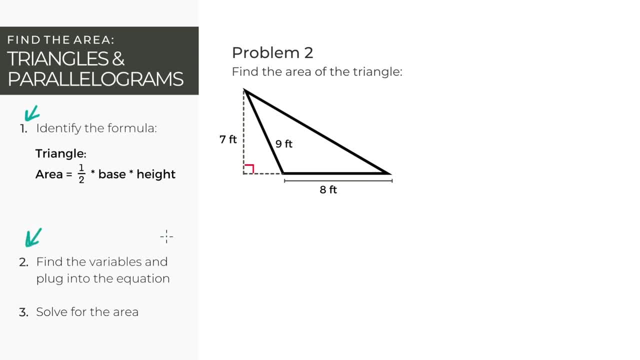 For the second step, let's figure out what the base and the height are for this specific triangle. The base is this side, the side that the triangle is sitting on, which is 8 feet, and our height, which is how tall the triangle is. 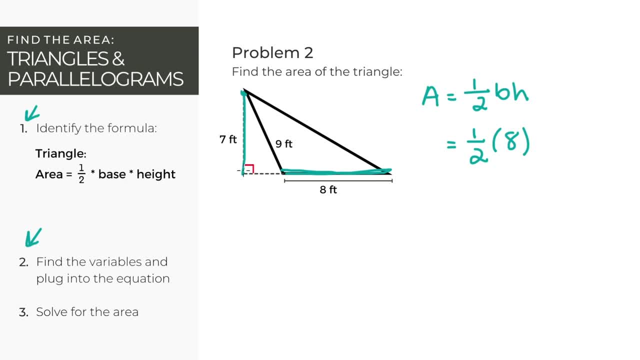 it's this line perpendicular or 90 degrees to the base, which is 7 feet, Even though this line isn't touching the actual base. that's okay. We're just measuring how tall the triangle is And don't get distracted by all of these other numbers. We only need the base and the height. 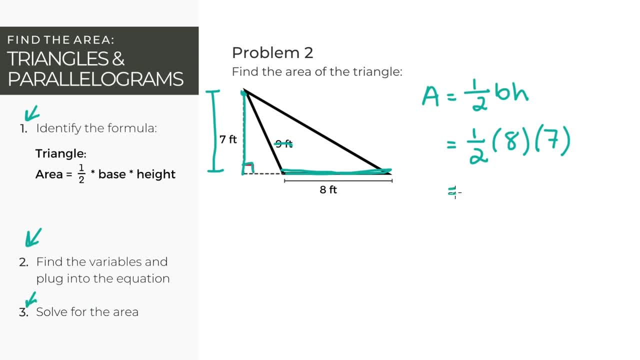 For our third step, we're solving the equation. We have that the area of the triangle is one half times the base, which is 8 feet, times the height, which is 7 feet. In solving the equation, we have that the area is 28 feet squared. 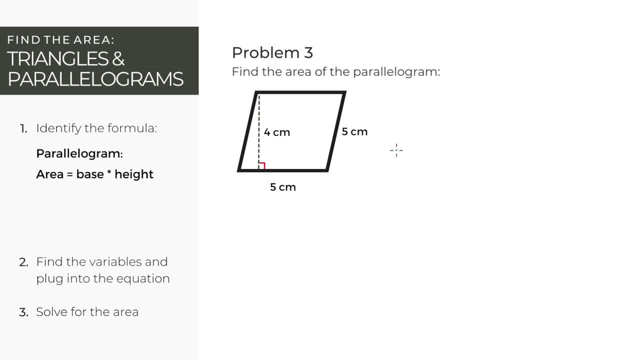 Let's now talk about parallelograms. We still have the same steps, but a different equation. Again, some person a long, long time ago discovered that the formula for the area of a parallelogram is just base times height. For step two, let's figure out what the values for the base and height are. 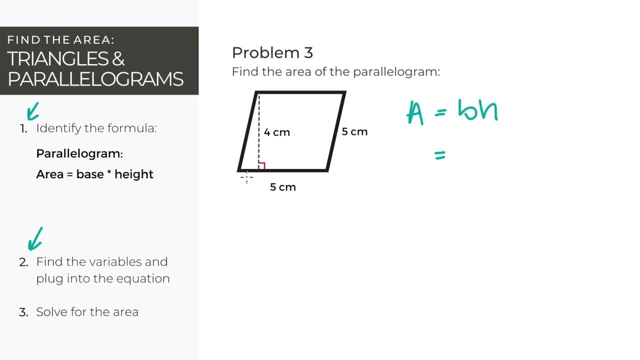 Similar to a triangle. the base of a parallelogram is the length of the side that it's just sitting on at the bottom here. Based off of this diagram, the base of this parallelogram is 5 centimeters, And the height, or how tall the parallelogram is, is the length of this line right here. 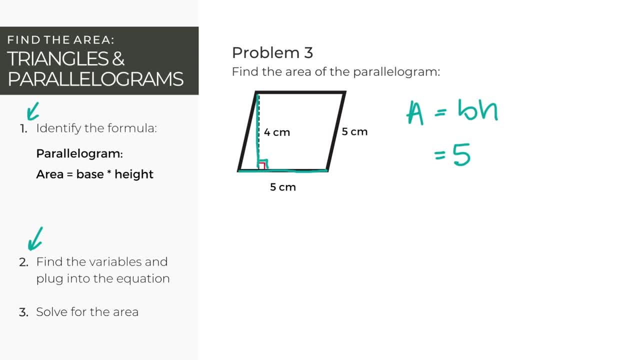 that is perpendicular, or in other words, 90 degrees to the base. Don't be fooled, it's not the length of this slanted one. It's this line running straight up and down, and in our case it's 4 centimeters. 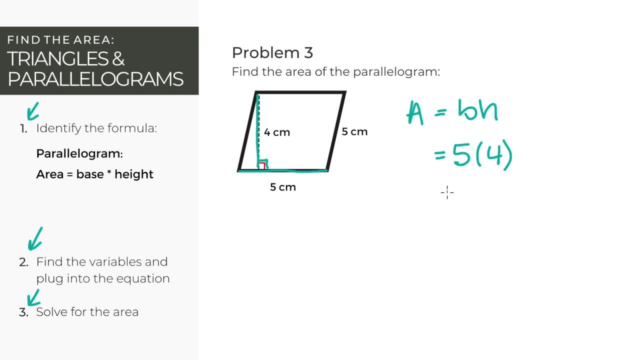 For our last step, let's solve the equation. The area of our parallelogram is the base, which is 5 centimeters times the height, which is 4 centimeters, and we'll get 20 centimeters squared. That's it. that's our answer. 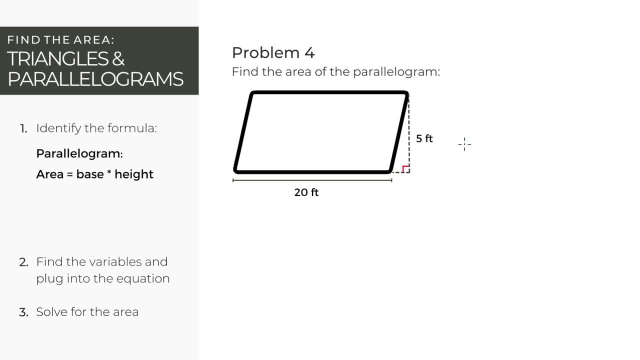 Let's do one more parallelogram example. For the first step, we're going to use the same formula, where the area of the parallelogram is base times height. Next let's figure out what the values for the base and the height are. 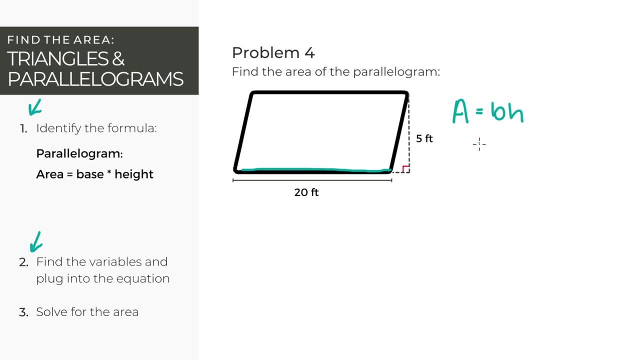 The base is this line here that the parallelogram is sitting on, which is 20 feet. The height of the parallelogram is this line, line here that is perpendicular, or in other words, 90 degrees, to the base, which is 5 feet. 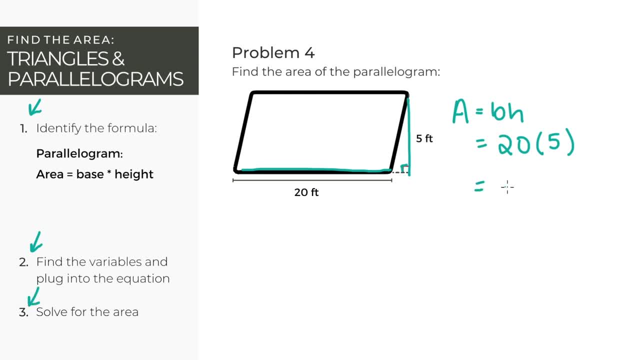 Finally, let's solve the equation and we'll get that. the area of this parallelogram is the base 20 times the height, 5, which is 100 feet squared. For our final area problem, let's get into one that's not as straightforward as the ones we've. 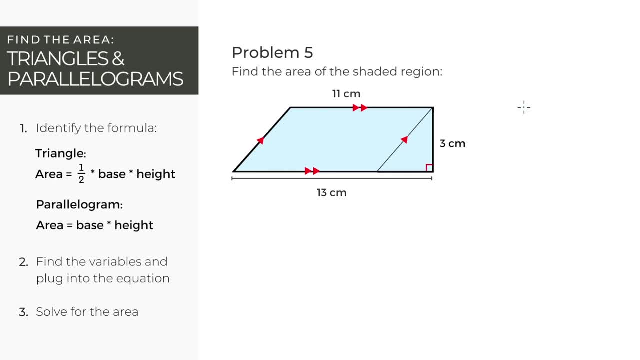 just seen. This shape isn't necessarily just a triangle or just a parallelogram, but if you look closely it's made out of a parallelogram and a triangle. We can see that this shape is a parallelogram because both sets of lines are parallel to each other and this shape is a. 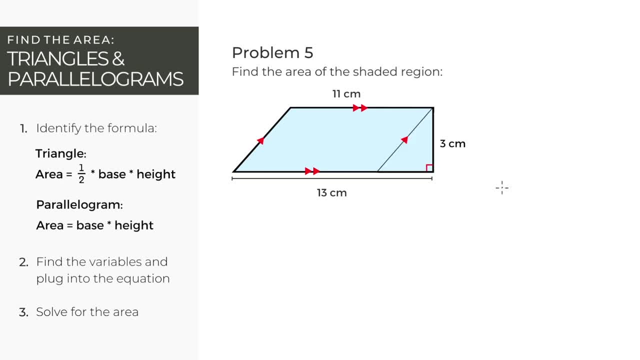 triangle. This shape looks like a triangle, doesn't it? So we can approach the problem in the same way, but we just have to do all of our steps twice, because this time we have both a parallelogram and a triangle. They're just attached to each other. 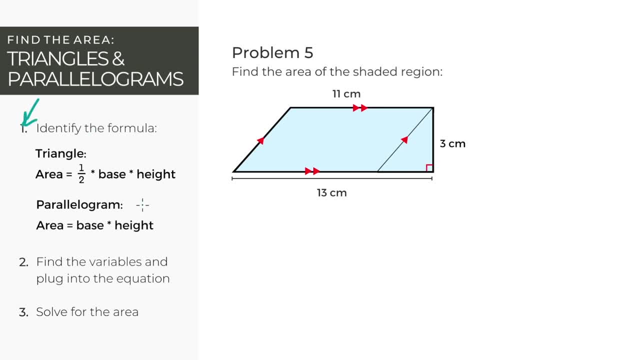 Let's do the parallelogram first. According to our formula, the area of a parallelogram is: base times height. The base of a parallelogram is the base times height. The base of a parallelogram is the base times height. The base of a parallelogram is the base times height. 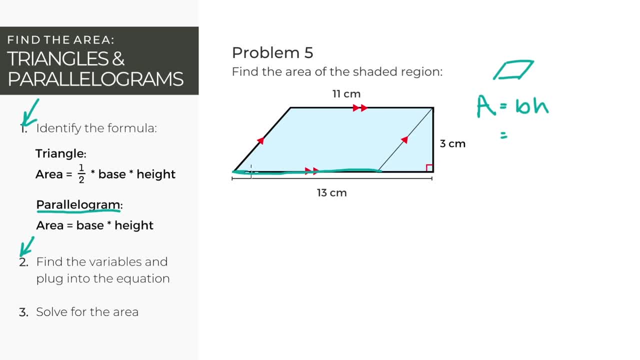 The base of the parallelogram is this line here. but be careful don't automatically plug in 13, because 13 is the length of this entire line. that includes the triangle part. The actual length of the base of just the parallelogram is 11 centimeters and I got this. 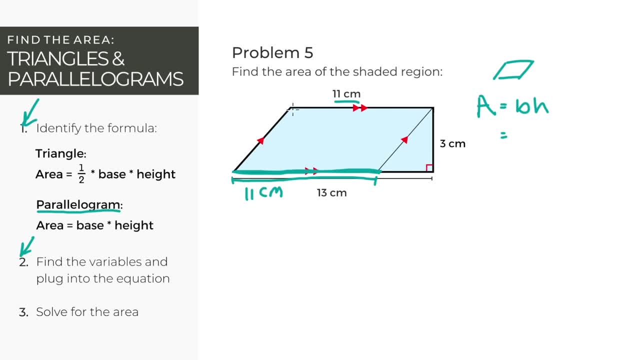 because it already tells us that this side of the parallelogram is 11 centimeters and just by the definition of a parallelogram, the lengths of these two lines are the same. These two sides are equal, so our base is also 11 centimeters. 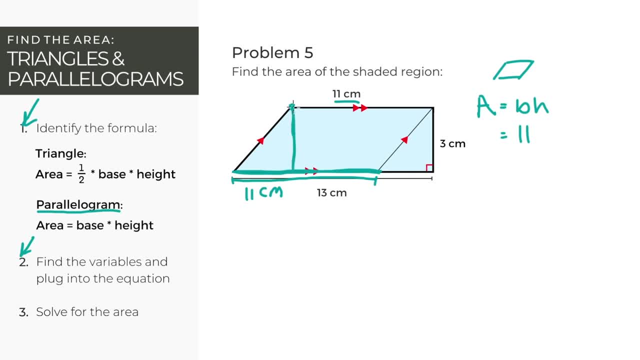 Now, the height of our parallelogram is this line that's perpendicular, or in other words, 90 degrees, to the base. You'll notice that this line is actually the same as this height we're given here, since it tells us that this line is also perpendicular to the base. 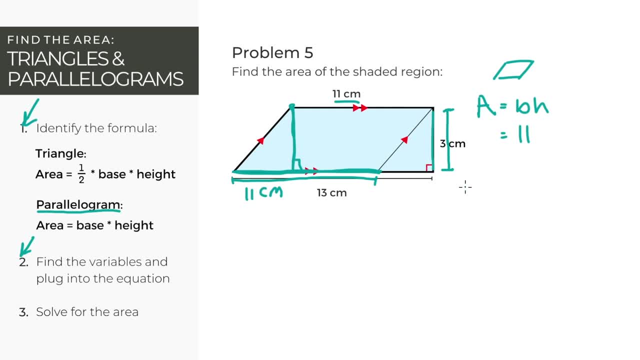 and it extends up to the top of the parallelogram. So the height of our parallelogram, based off of this diagram, is three centimeters. Solving for the equation now we get that the area of the parallelogram is the base, which is 11 centimeters times the height, which is three centimeters.